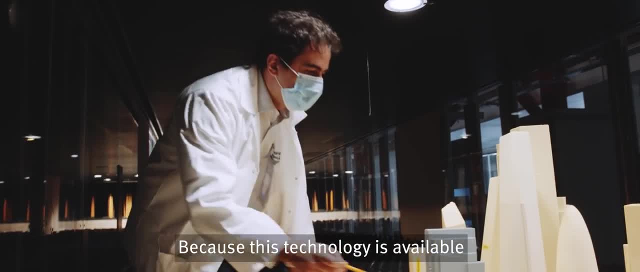 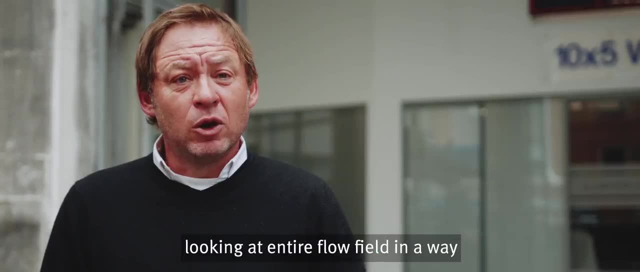 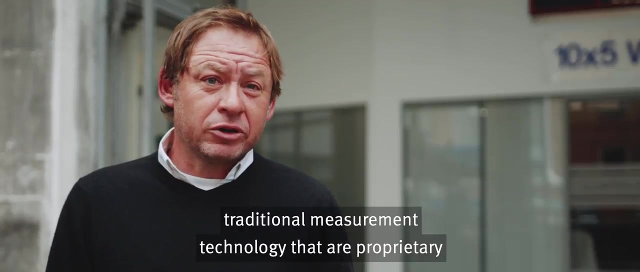 We've got a new wind tunnel. We've got a new wind tunnel. This is a new wind tunnel. This is a new wind tunnel. We have a new facility which is what makes it ideally suited for our work. Because this technology is available to us here in this facility, we can now take it to looking at wind flows around buildings and large-scale structures, looking at entire flow field in a way that we would not have been using traditional measurement technology that are proprietary to the wind engineering sector. 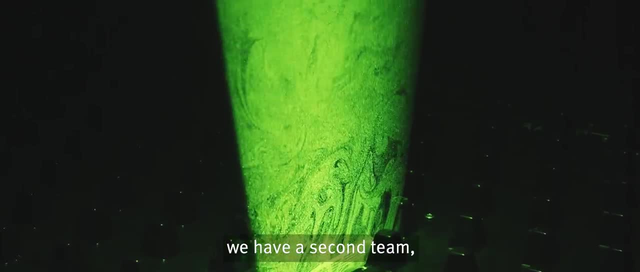 Simultaneously, more upstream, in the lower section, we have a second team. They're setting up a particle image velocimeter. 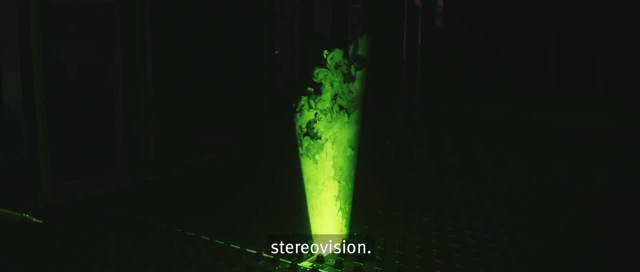 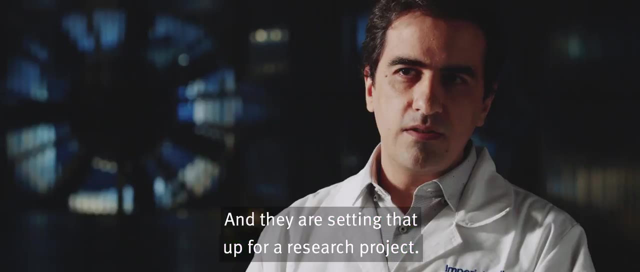 system, a PIV system, laser-based diagnostics, stereo vision, so it gives them three components UVW of velocity in a time-resolved fashion and they are setting that up for a research project. 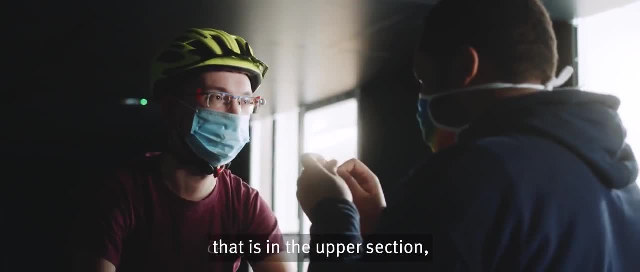 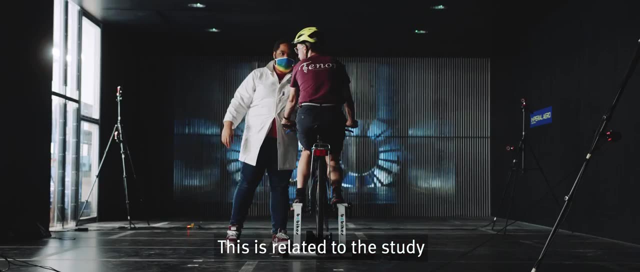 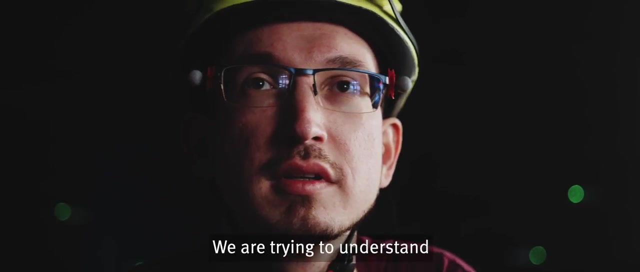 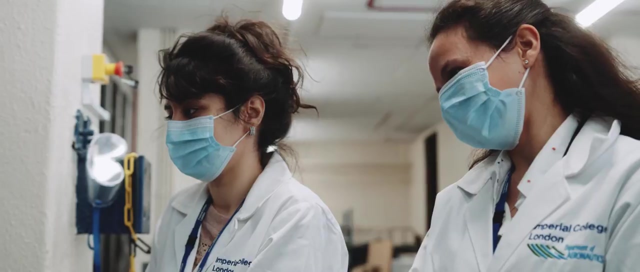 We have a third team that is in the upper section and they are setting up a cycling rig. This is related to the study of transmission of SARS like viruses. We are trying to understand and provide guidelines of what is safe social distancing while people are doing sports. 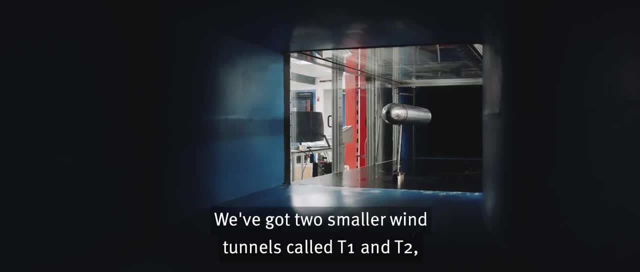 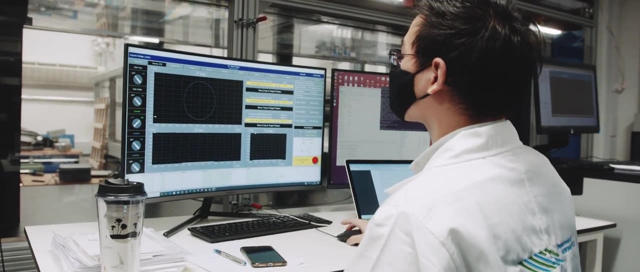 We've got two smaller wind tunnels called T1 and T2, one square meter cross-section and about two square meter cross-section. We've got a flume, that's a water tunnel. 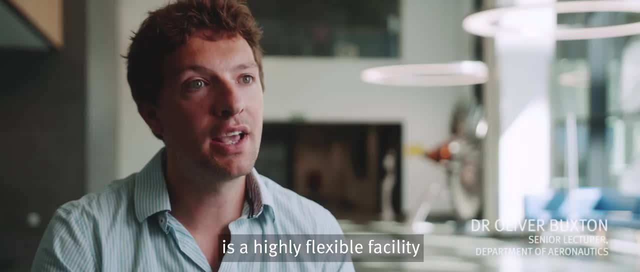 So our field is a water tunnel. We have a water tunnel that is a water tunnel. So our field is a water tunnel. We have a water tunnel that is a water tunnel. So our flume here at Imperial College London is a highly flexible facility which is 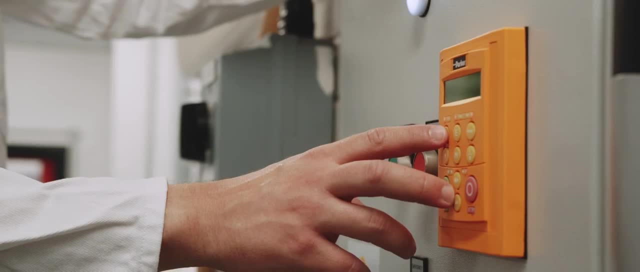 well optimized to make measurements of both velocity and scalar. We can do very similar experiments in our flume that we can do in the wind tunnels, except 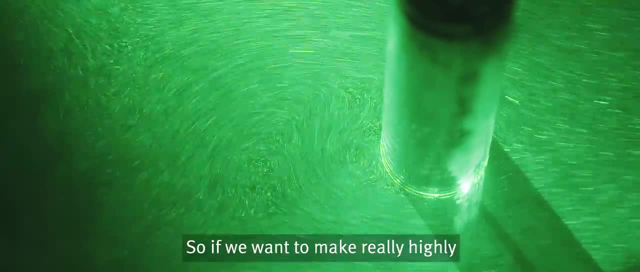 effectively we've slowed everything down by ten times. So if we want to make really highly temporally resolved measurements then the flume is perfect. 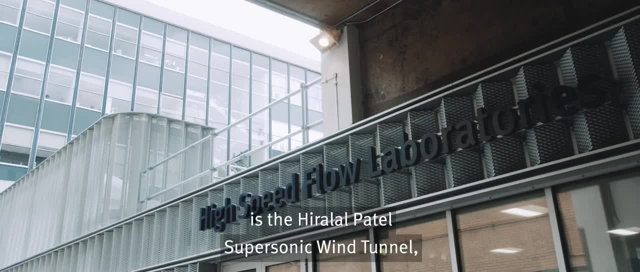 One of our newest most advanced facilities is the Hiralal Patel supersonic wind tunnel, which has a unique range of operating capabilities up to Mach 4. 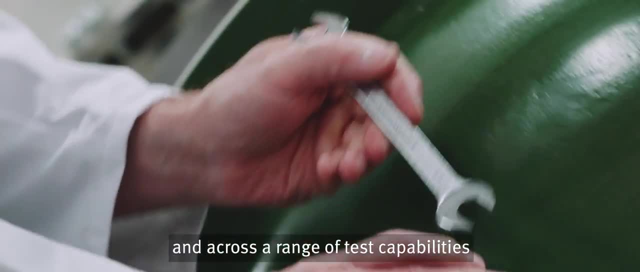 And across a range of test capabilities which allow us to model everything from satellites re-entering the Earth's atmosphere to high-speed ejection tests. 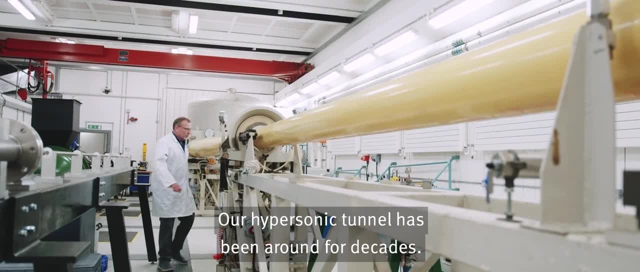 Our hypersonic tunnel has been around for decades and for the last 50 years it's really been at the forefront of some of the pioneering advances in hypersonics 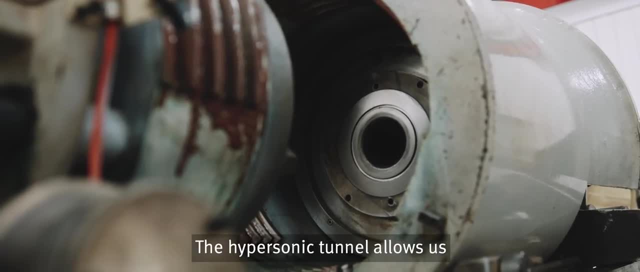 aerodynamics and that's still the case today. The hypersonic tunnel allows us to test objects up to Mach 9. 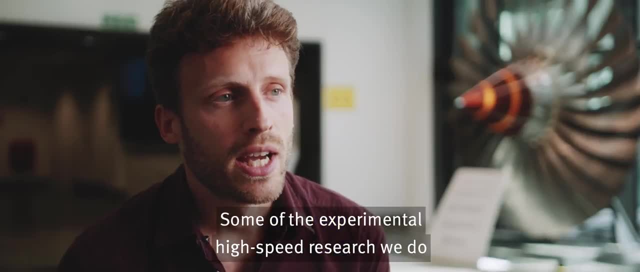 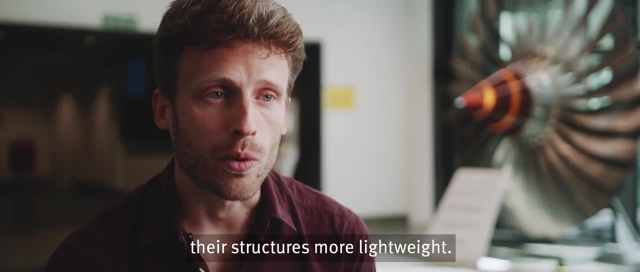 Some of the experimental high-speed research we do looks at the inter- action between flexible structures in high-speed flows. So more and more designers are making their structures more lightweight and as you make a structure lightweight it becomes more flexible and how that interacts with the high-speed aerodynamics is a real challenge for designers. 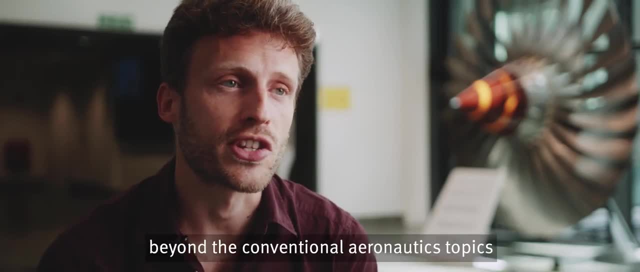 So one topic we're interested in that's a little bit beyond the conventional 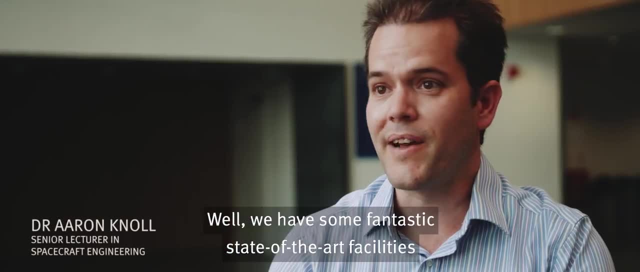 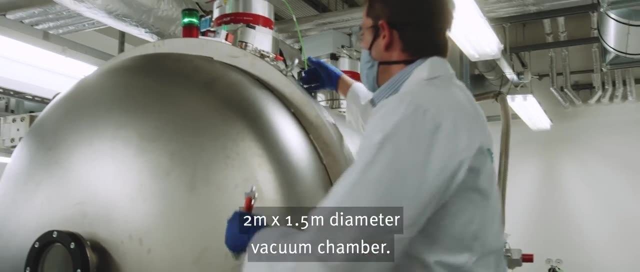 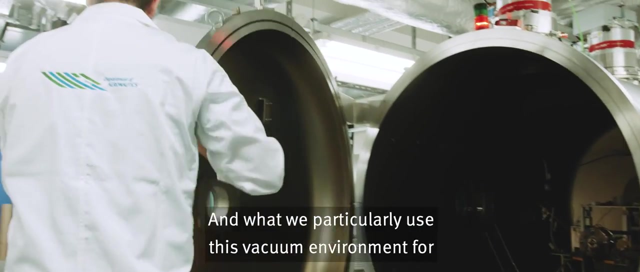 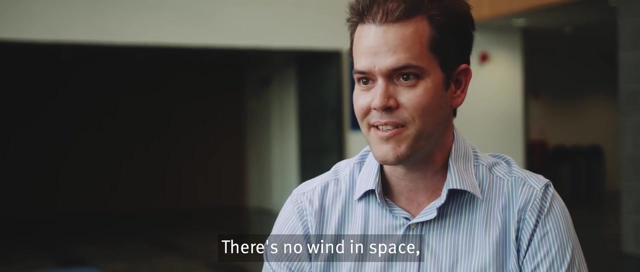 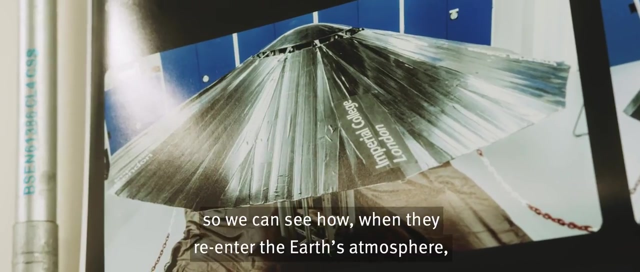 aeronautics topics is access to space. Well we have some fantastic state-of-the-art facilities in the space research lab. So one of those is a large 2 meter by 1.5 meter diameter vacuum chamber. So this replicates the conditions of being in space and what we particularly use this vacuum environment for is to test our spacecraft propulsion systems. There's no wind in space but what we use the supersonic wind tunnel for is testing re-entry vehicles so we could see how when they re-enter the Earth's atmosphere exactly how they behave and the characteristics of the flow field around them. 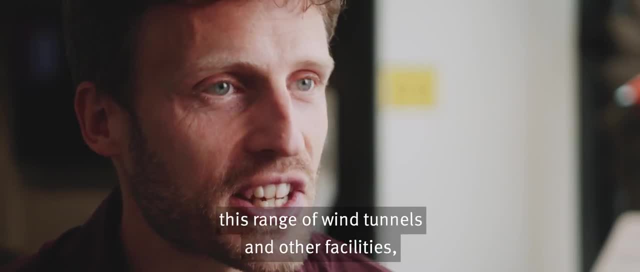 So the Department of Aeronautics brings together this range of wind tunnels and other facilities and the personnel to run them to really create a center for excellence for aerodynamics research. 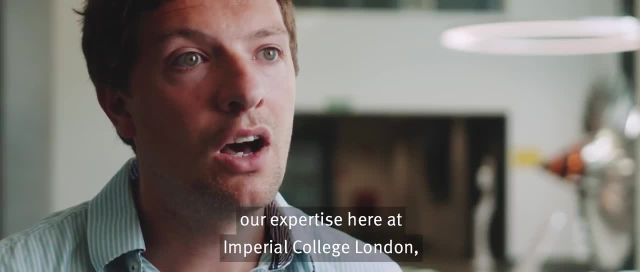 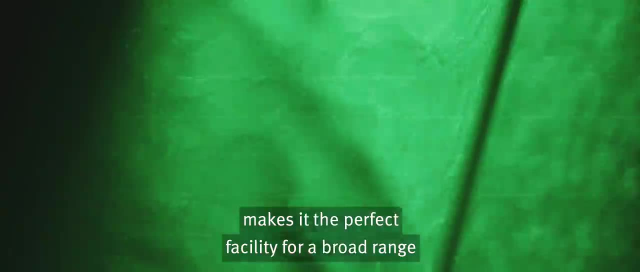 Well the combination of the design of the facility, our expertise here at Imperial College London and the equipment that we have in terms of the high-speed lasers and cameras makes it the perfect facility for a broad range 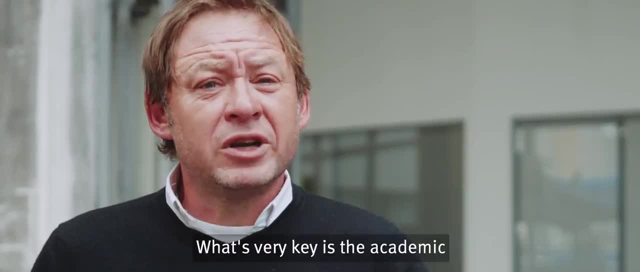 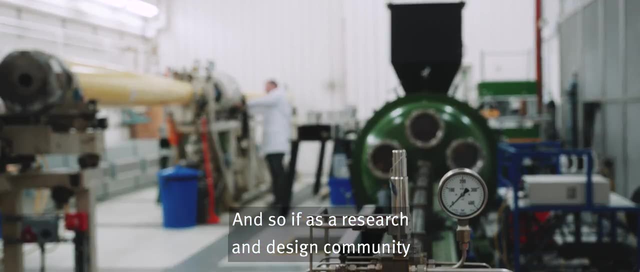 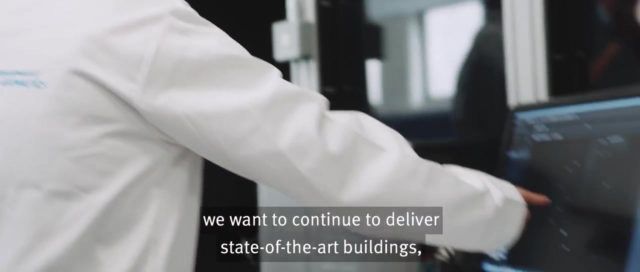 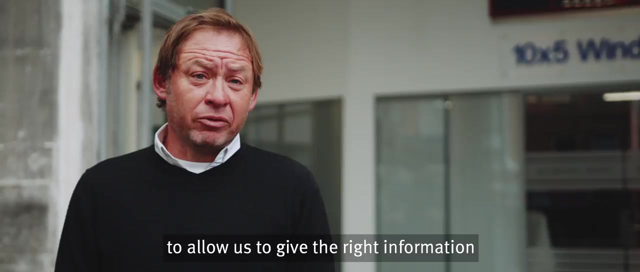 of experimental fluid mechanics applications. What's very key is the academic and technical support that we get with this facility and so if as a research and design community we want to continue to deliver state of the art buildings we need cutting-edge facilities such as the 10x5 wind tunnel facility to allow us to give the right information to designers in the technical detail that they needed.